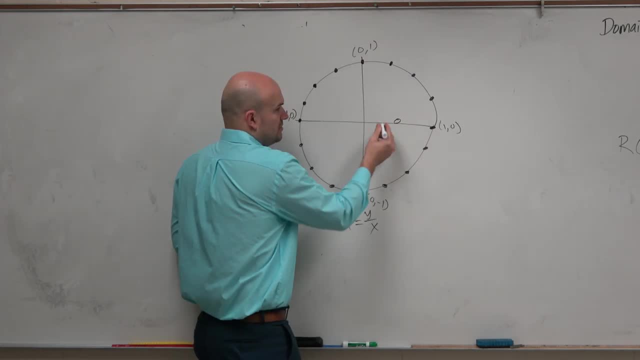 What are the angles here that I have Remember the first angle would be 0.. This angle is pi halves And this angle is pi halves. This angle is pi. This angle is 3 pi halves And that angle is 2 pi right. 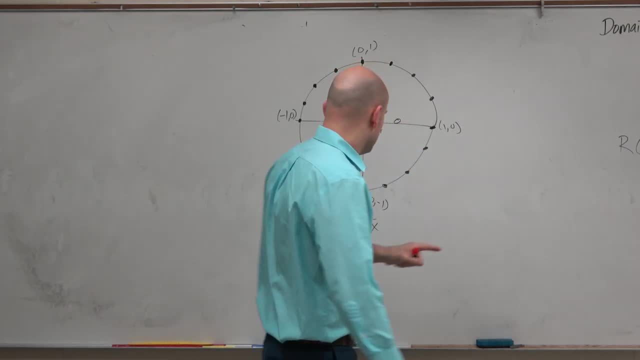 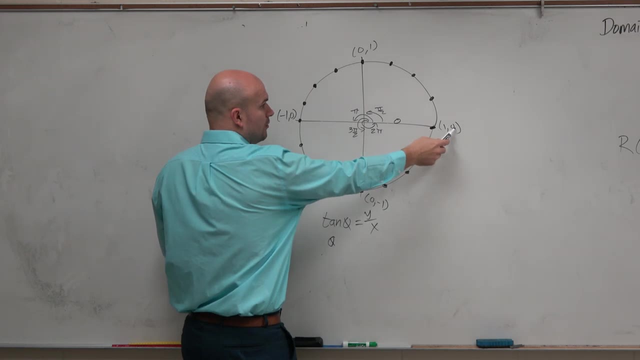 So what is the first angle of tangent? Let's figure that out. The first angle. so when I say, when theta equals 0, is tangent undefined. y over x, No, OK, cool. So asymptotes, What about at pi halves? 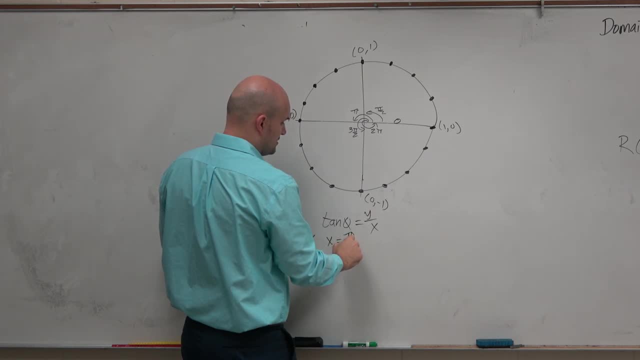 Yes. so I could say my asymptote occurs: at x equals pi halves. What about at pi No? What about at 3 pi halves? Yes, OK, x equals 3 pi halves, And then at 2 pi No, right. 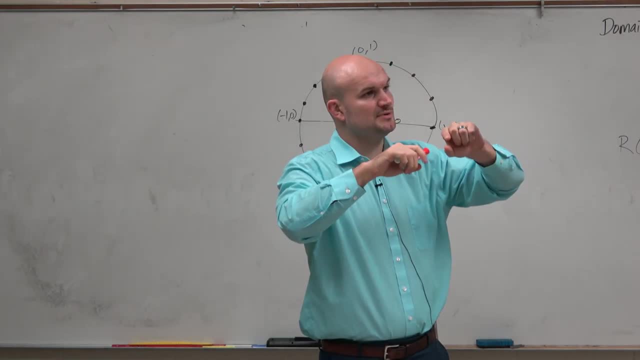 But then what we looked at. if you guys remember when we did, if you guys remember the Desmos, I showed you that one where you go around the unit circle and then it plots the sine graph, right, And then I said, guys, we're not restricted. 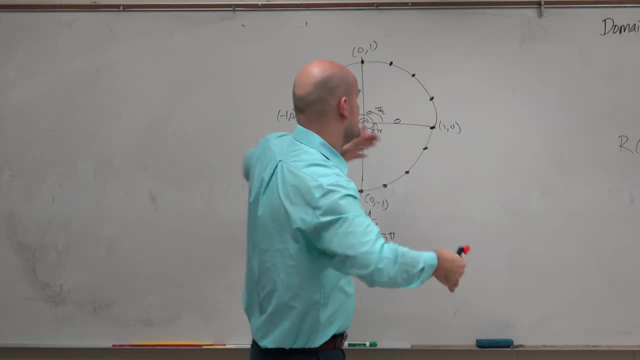 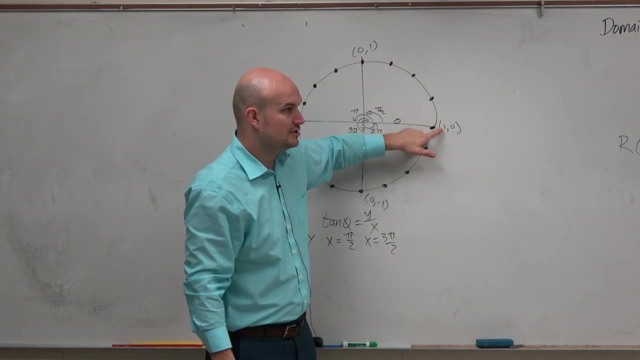 to going around the circle once. We just practice going around the circle once to identify the initial period so we can look at what that graph looks like. But in reality we know, So you can go around the circle once. You can go around. 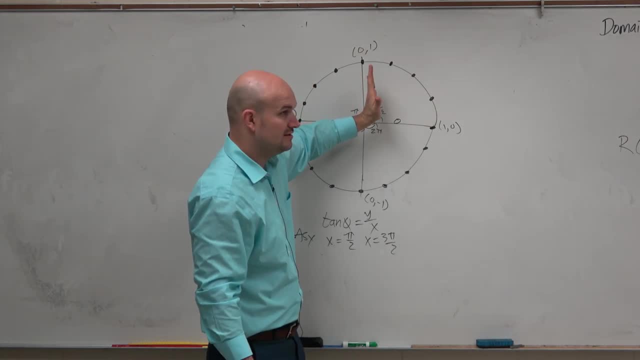 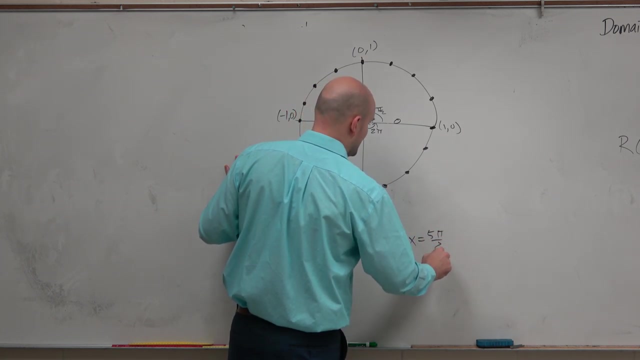 And then. so, as you go around again, the next asymptote is going to be 5 pi over 2.. And then you're going to get to 7 pi over 2.. And you can keep on going and going. So as this goes, x equals 5 pi over 2.. 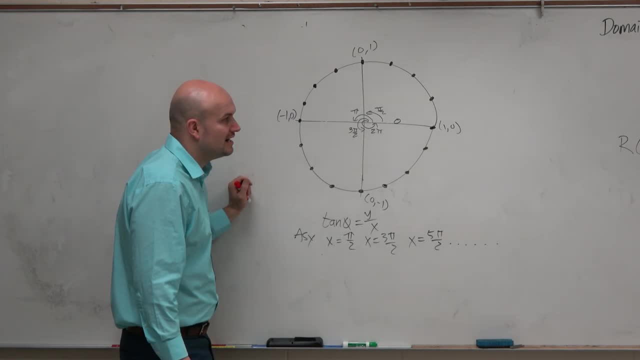 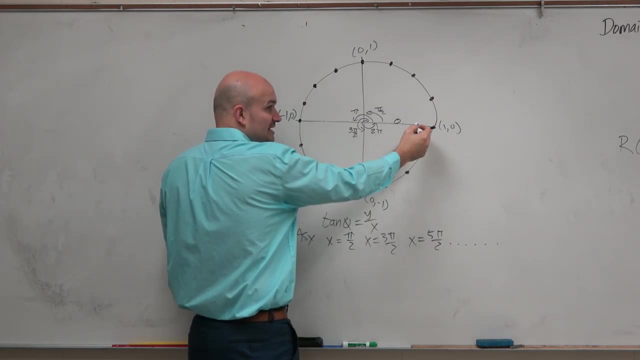 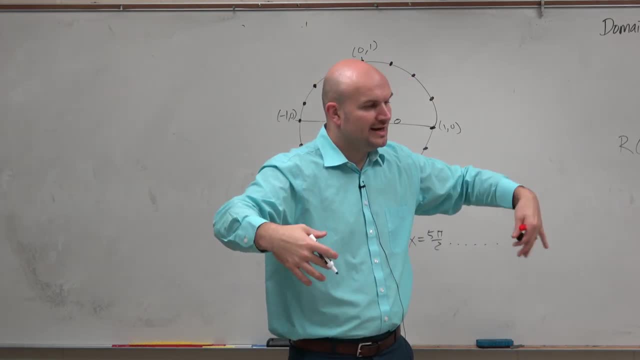 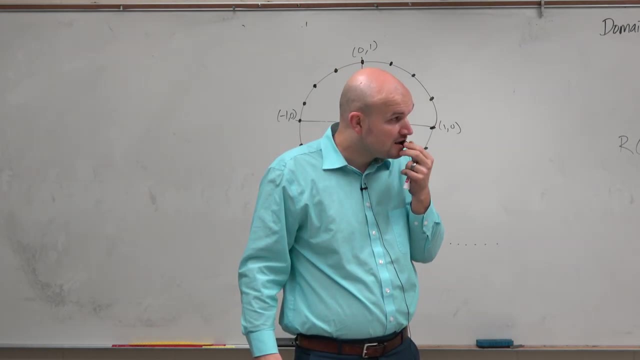 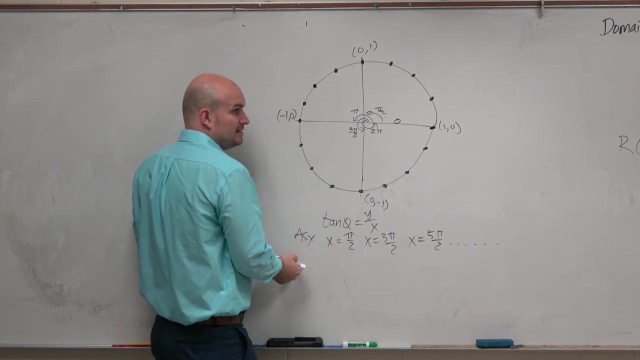 So, rather than trying to memorize all these asymptotes, we also know that it's impossible to write them all, because there's infinite many. Yes, It's when 0 is in the denominator. Tangent is the y-coordinate over the x-coordinate. 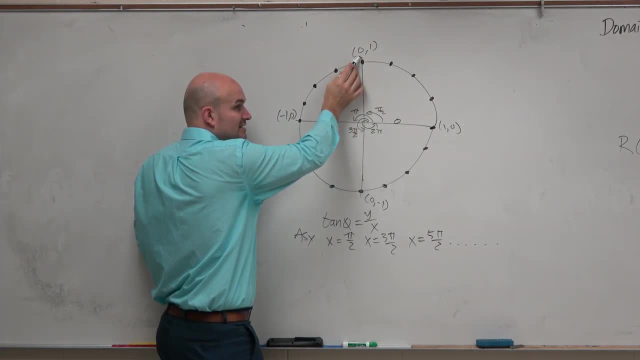 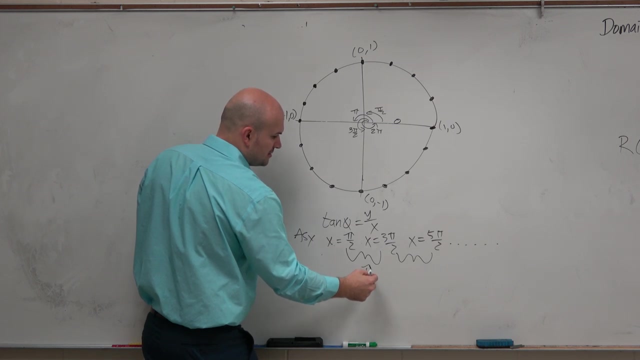 At pi halves. my y-coordinate is 1.. My x-coordinate is 0.. 1 over 0 is undefined. So then we start to look at. well, what patterns then can we figure out From pi halves to 3? pi halves is plus pi. 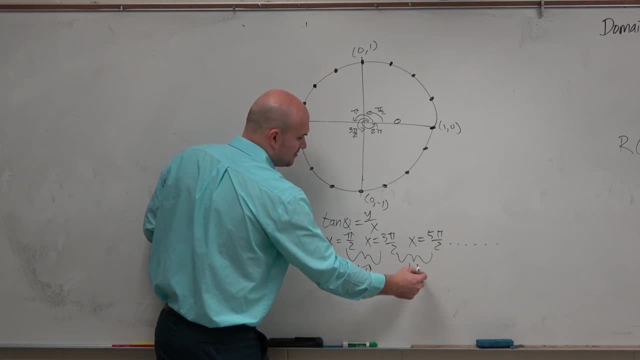 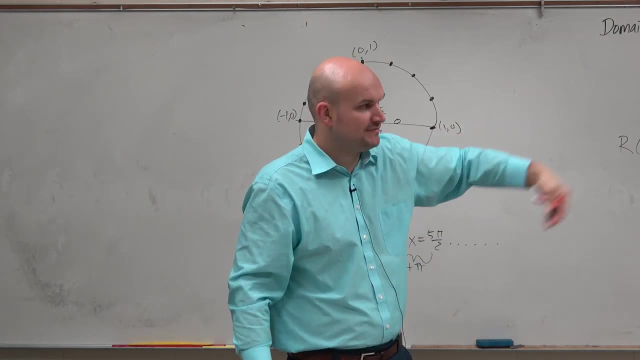 From 3 pi halves to 5 pi halves is plus pi. And if we keep on going, we see that if we just keep on adding pi, we're just going to keep on getting asymptote after asymptote after asymptote after asymptote. 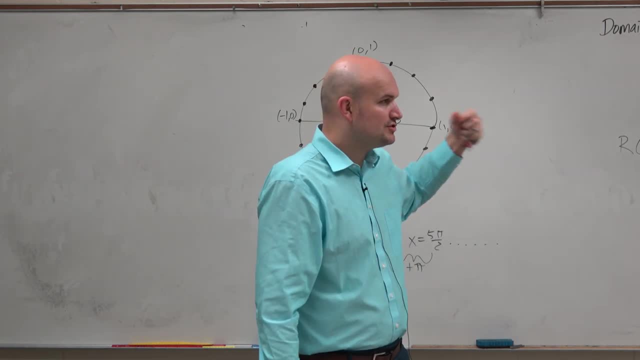 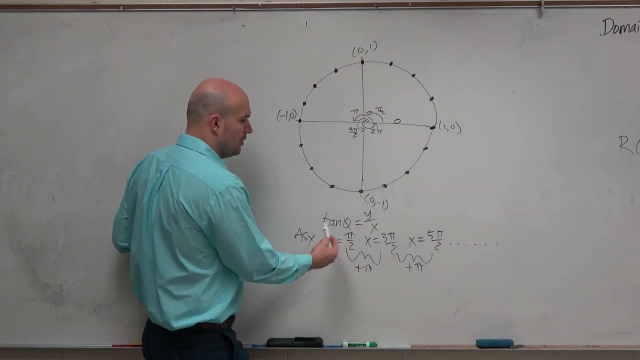 Right. So if we keep on adding pi, we're just going to keep on getting asymptotes. So, rather than trying to list the asymptotes, we can write an equation that represents all of the asymptotes, And so what we do is, rather than just like saying this, 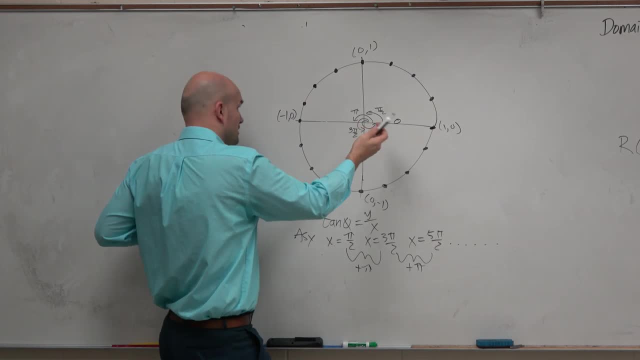 we know that to you. And again, you can look at it this way as well: As you get to pi, halves the distance to the next asymptote, is halfway around the circle, which is pi. And then if you add pi again and then add pi again, 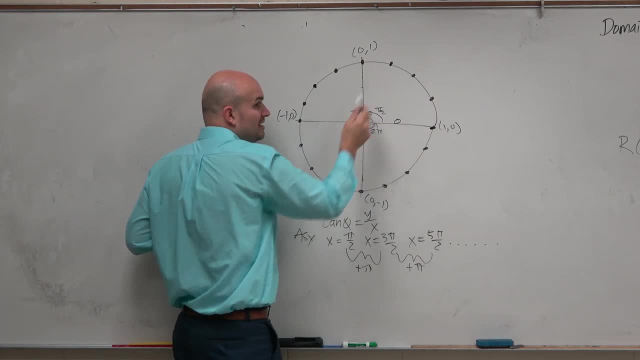 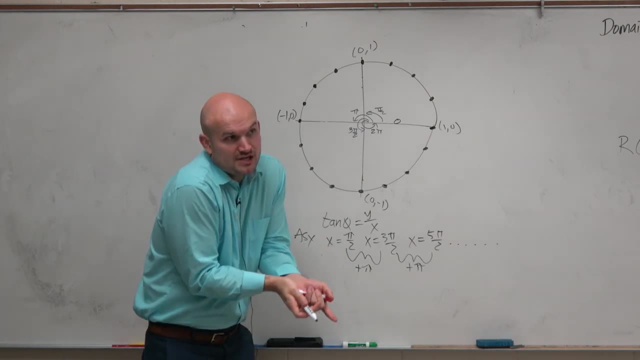 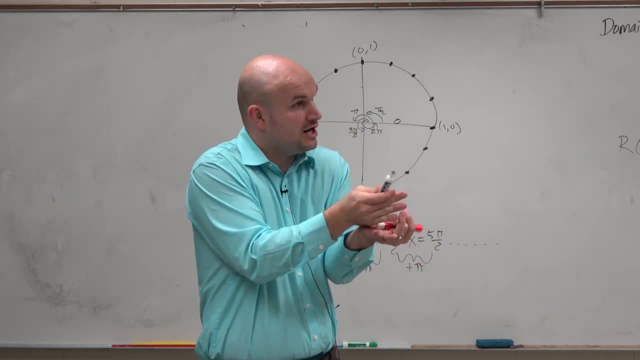 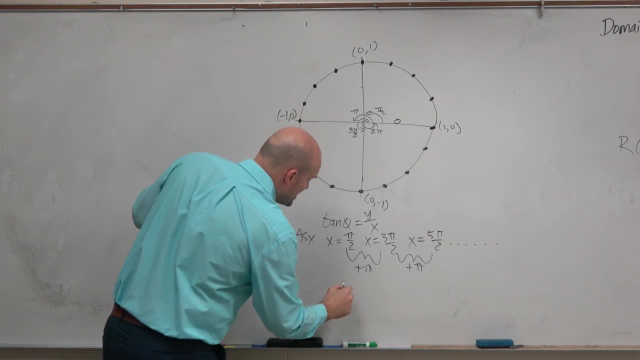 And again, you can start any asymptote, As long as you know what one asymptote is. start there. Typically on a multiple choice test, they're going to provide the smallest positive as your asymptote. So we would say x is equal to pi halves. 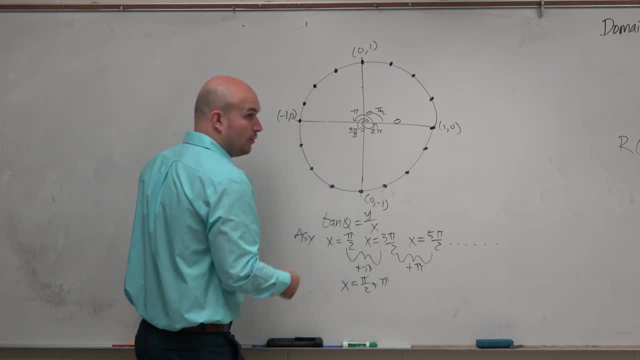 And then to get to the next one, I'm going to have to add or subtract pi, But to represent the adding and subtracting we're going to use n. So we'd say: x equals pi, halves plus pi n, And that is the equation for the asymptote for tangent. 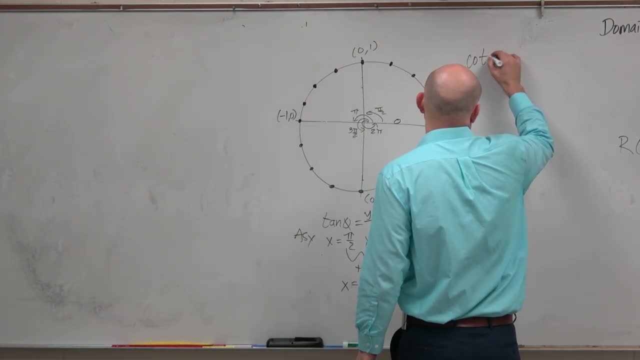 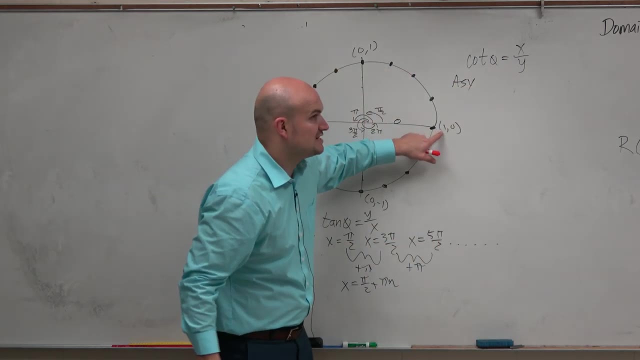 Now let's go and look into cotangent. Cotangent theta is x over y And if we look at the asymptotes- in this case, this is when it's the x-coordinate over the y-coordinate- And we see there's an asymptote at x equals 0.. 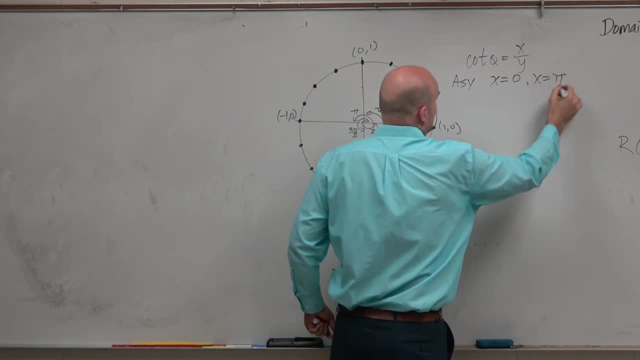 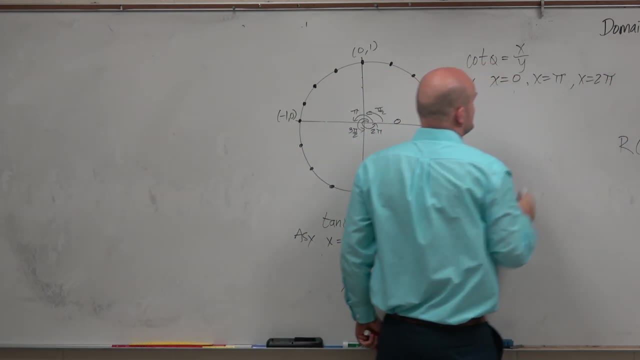 No, And at x equals pi. And again, if we notice this- 0 to pi, the next one is going to be It's going to be at 2 pi. So the smallest positive asymptote I have is 0.. 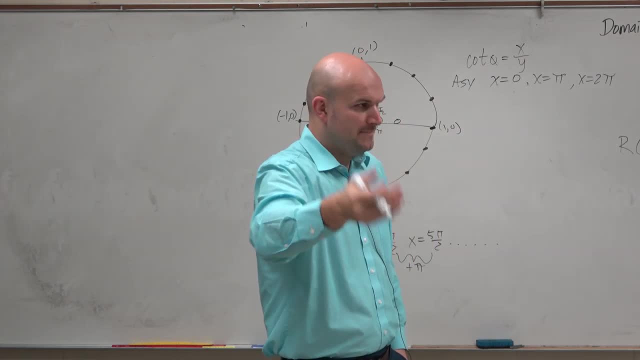 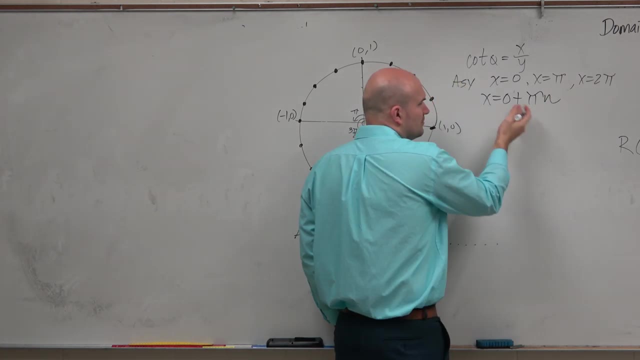 And then the distance between each asymptote is again pi. But to go positive and negative we're going to use pi? n. So we'd say x equals 0 plus pi n. Well, we don't really need to write the 0 there. 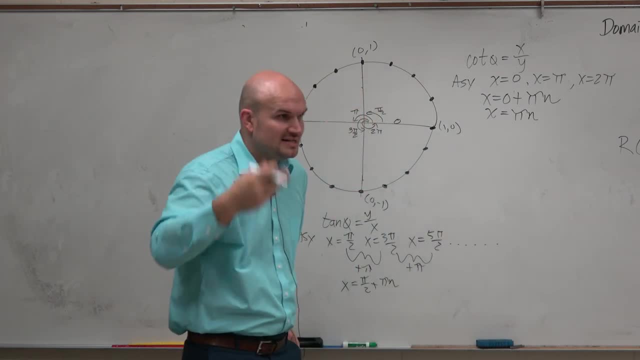 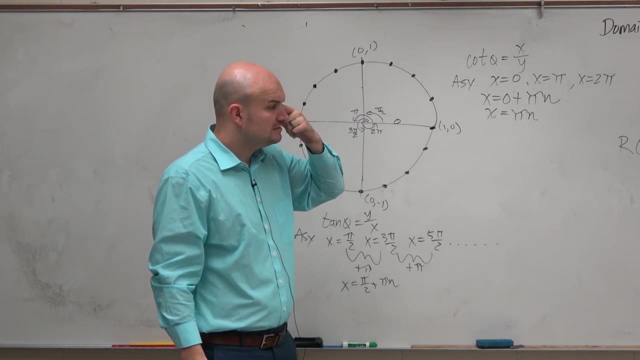 So we can just say x equals pi, n. I'm not memorizing anything, I'm just looking at four coordinate points on the unit circle to understand where my asymptotes are. Yes, When we write asymptotes, do you want them to be? 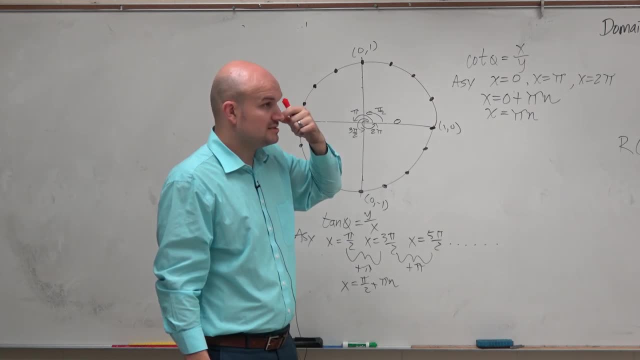 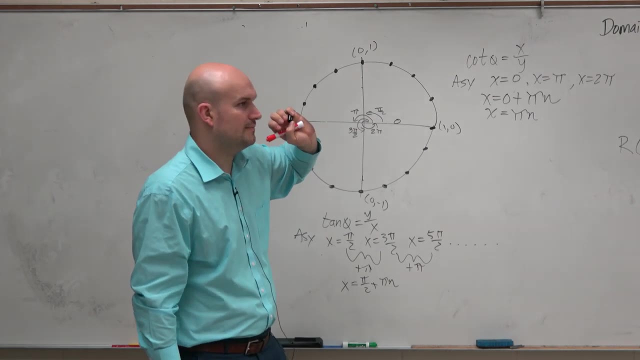 on the straight: x does not equal or x does equal, x does equal. If it's in the domain, then those are undefined values, But x equals is the correct version for that. Now let's go and look at our other two functions. 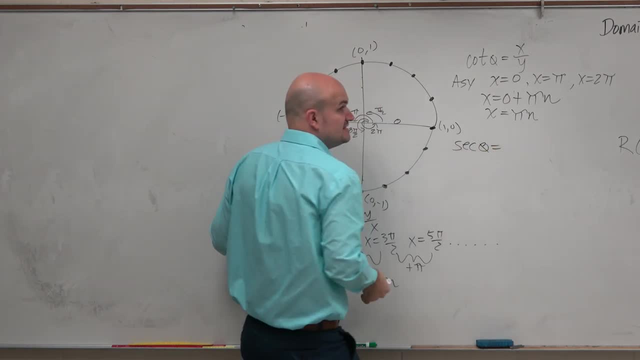 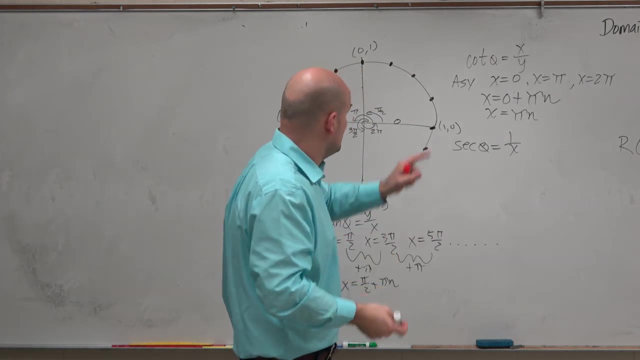 Secant, Secant of theta. Secant of theta is 1 over x. So basically, here we're looking for. well, when is the x coordinate going to be 0?? Nope, not, there Is the x-coordinate here. 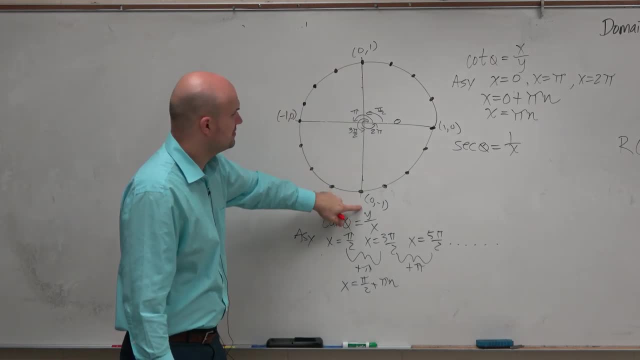 So, again, at pi halves. It's undefined, Defined, Oh, undefined, Oh, wow, Undefined. at pi halves, undefined at 3 pi halves. That looks very similar to the tangent one, right. So to save myself some time, I'm just: 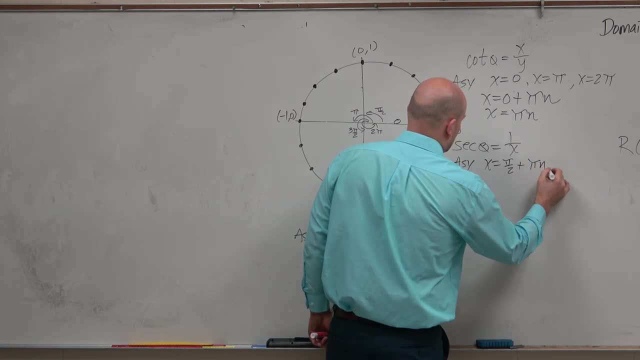 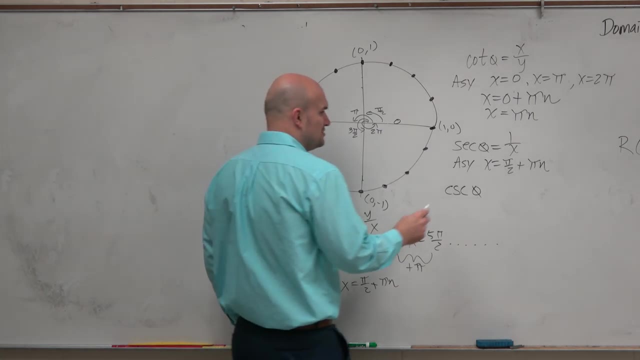 going to write: x equals pi halves plus pi n, And then, if you've figured out any sort of relationship so far, you'll realize that cosecant of theta is going to be the same as cotangent. But let's just not believe that. 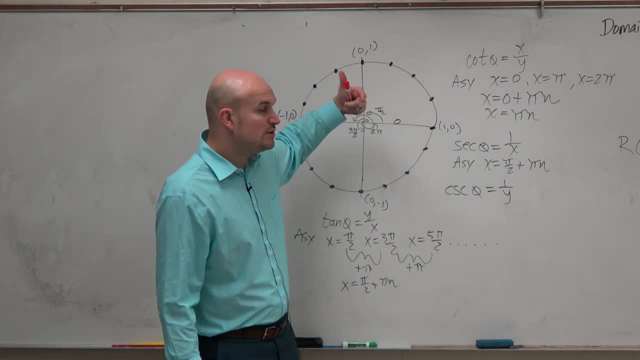 Let's actually check it. Cosecant has asymptotes. What happens when y is 0? 1 over 0? Yep, that's at 0.. Nope, Yep, Oh, it's 0 and pi 2, pi, 3, pi 4, pi 5, pi 6, pi, negative, pi, negative, 2, pi. 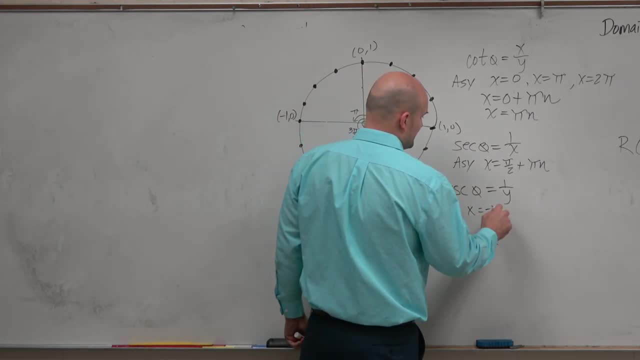 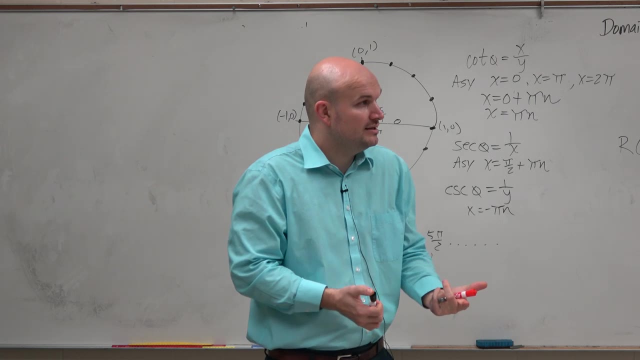 negative 3 pi. negative 4 pi. So I would just say x is equal to negative pi n. So those are my asymptote equations: right, And it's all finding good when we don't have any transformations left or right. right. 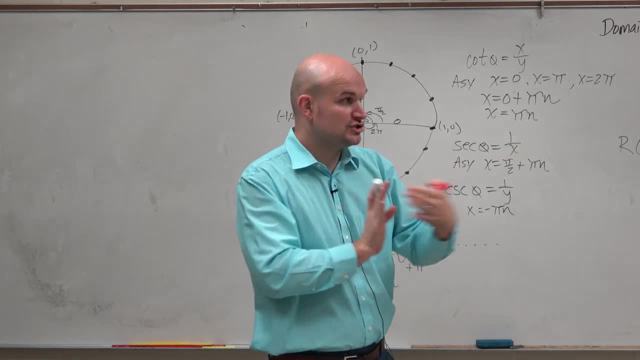 Because if I don't have any shifting left or right, stretching or compression or whatever, I'm just going to say if I don't have any compression or shifts, then those are what my asymptotes are And it's really easy to get them.